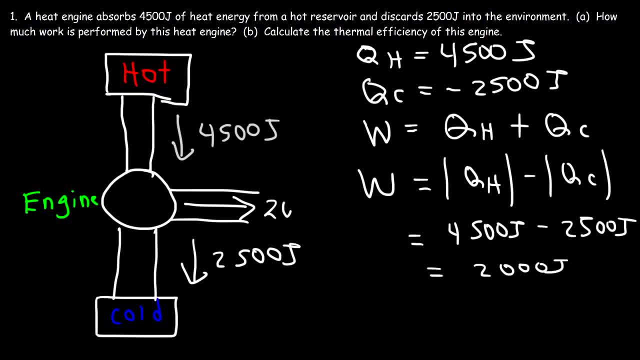 converted to mechanical work, it's 2,000 joules of heat energy and this makes sense. the engine absorbs a total of 4,500 joules of heat energy and then it releases 2,500 joules and 2,000 joules. if you add 2,500 and 2,000, that's 4,500. 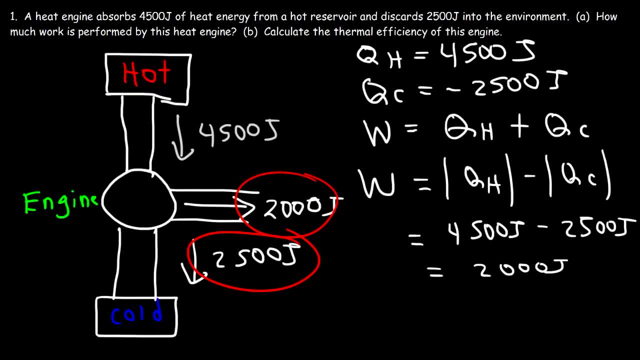 joules. so if 4,500 joules of energy goes into the system, in order for the system to maintain its temperature it has to release 4,500 joules of energy. so the amount of energy that comes into the engine must equal the total amount of 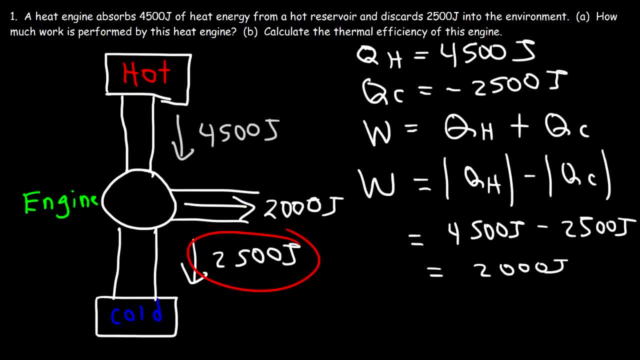 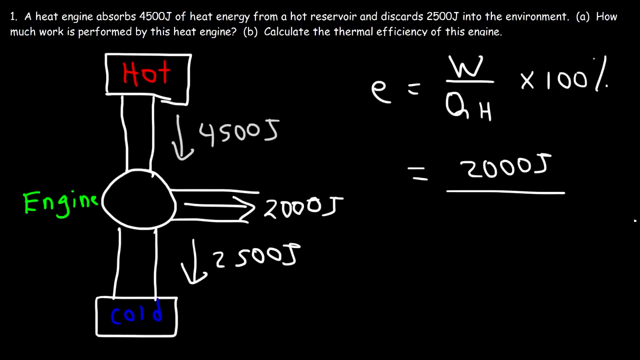 energy that leaves the engine so that it can maintain its original state. now let's move on to Part C: calculate the thermal efficiency of this engine. the thermal efficiency is the mechanical work divided by QH, multiplied by 100%. so in this example the mechanical work is 2,000 joules, the amount of heat energy that was absorbed. 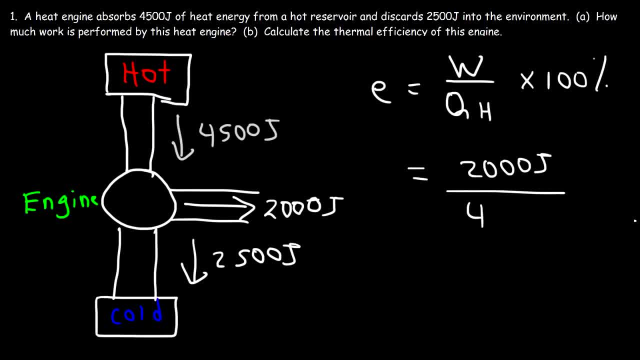 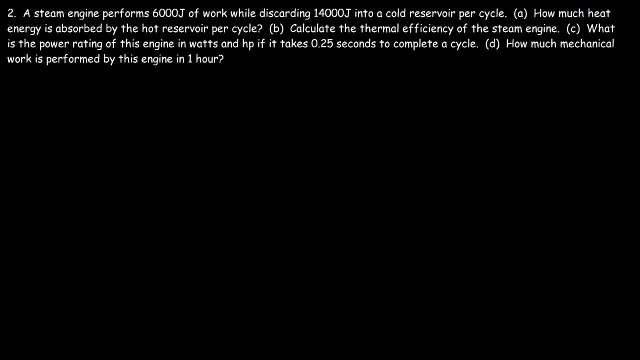 by the hot reservoir per cycle is 4,500 joules, and then we need to multiply this by 100%, and so the efficiency in this example is 44.4 percent, and so that's the answer to this problem. now let's move on to number two. a steam engine performs. 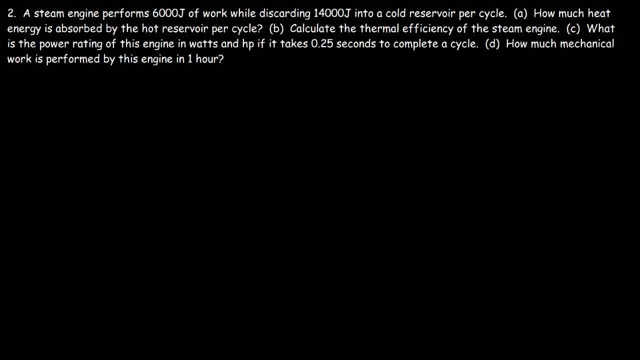 6,000 joules of work While discarding 14,000 joules into a cold reservoir per cycle. How much heat energy is absorbed by the hot reservoir per cycle? So let's draw a picture. So here we have our energy flow diagram. 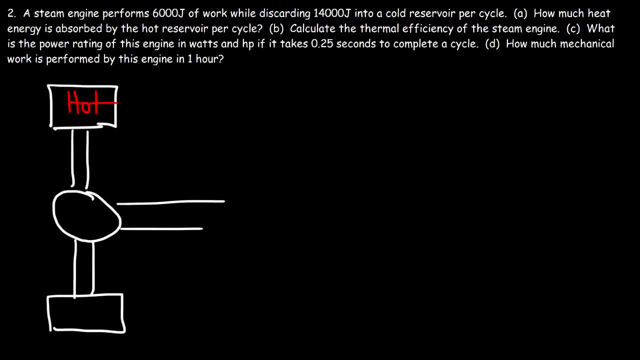 And so this is going to be the hot reservoir, just like before, And this is going to be the cold reservoir. So 6,000 joules of mechanical work is being performed. So that's W. So we have that, And the steam engine discards 14,000 joules into the cold reservoir. 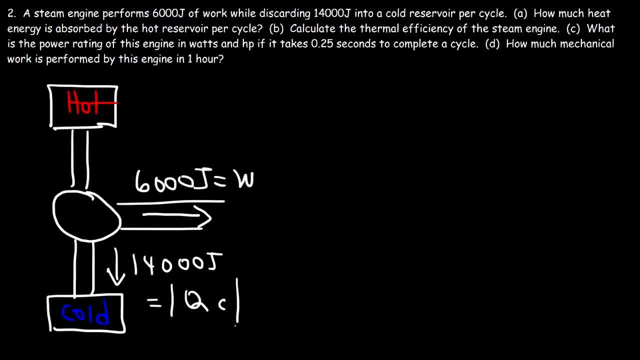 So that's the absolute value of Qc. Qc is negative 14,000.. How much heat energy is absorbed by the hot reservoir per cycle? So we're looking for Qh. So we know that W? W is the absolute value of Qh minus Qc. 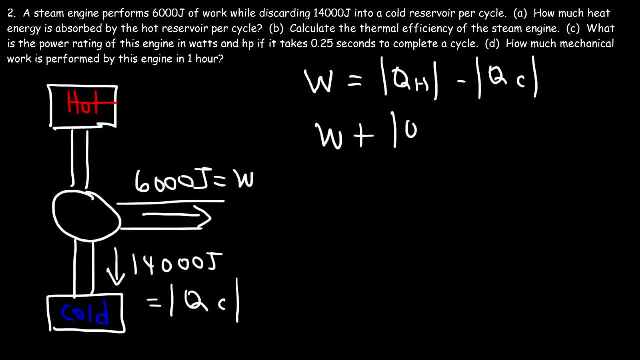 So Qh is going to be W plus the absolute value of Qc, And Qh is going to be positive. So W in this example is 6,000 joules And Qc is 14,000 joules, So Qh is going to be 20,000 joules. 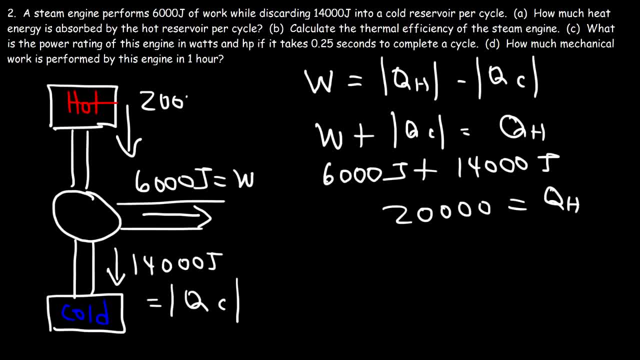 And so 20,000 joules of thermal energy Is taken from the hot reservoir per cycle. Part B: Calculate the thermal efficiency of the steam engine. The thermal efficiency- just like before it's going to be the work divided by Qh times 100%. 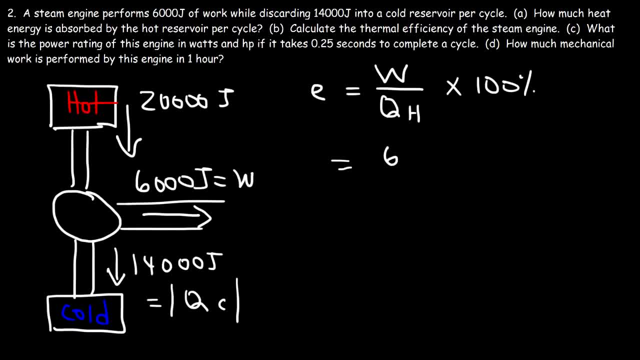 So the work output is 6,000 joules, Qh is 20,000.. And let's multiply that. Multiply that by 100.. So the efficiency in this example is 30%. So that's the answer for Part B. 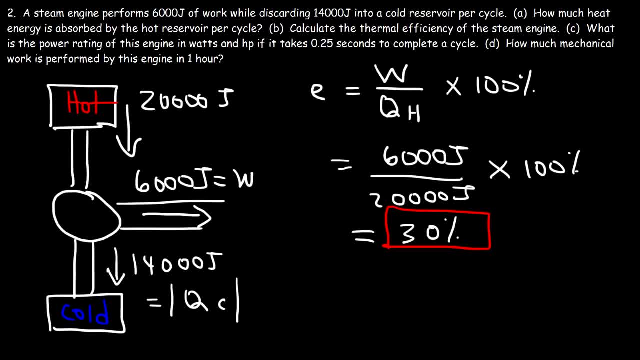 Now let's move on to Part C. What is the power rating of this engine in watts and also in horsepower, if it takes 0.25 seconds to complete a cycle? So how can we calculate the power? Power is work divided by time. 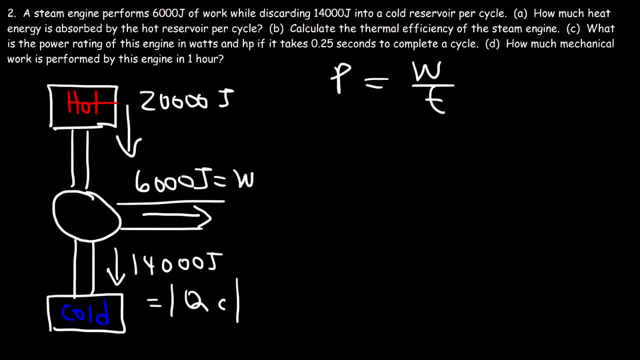 And so we have the work. It's 6,000 joules per cycle. However, we have the time it takes to complete a cycle- Watts. I mean work is in joules And time is in seconds. So 1 joule per second is equal to 1 watt. 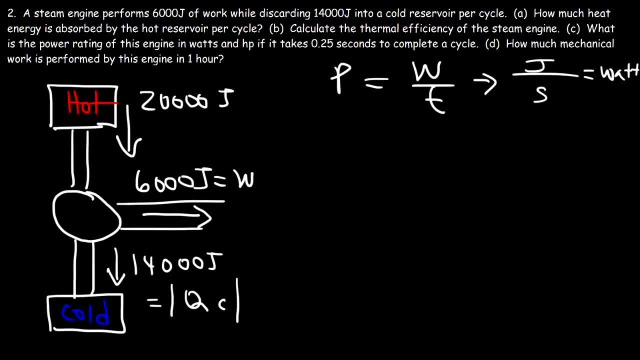 Which is the unit for power. So keep that in mind. Now, what I'm going to do is start with this value. The work output is 6,000 joules per cycle, So in two cycles, the machine or the engine will do 12,000 joules of work. 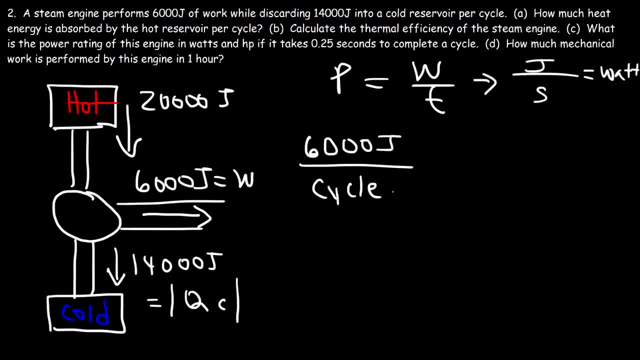 In three cycles: 18,000.. In four cycles: 24,000.. So every cycle that the machine goes through, 6,000 joules of mechanical work will be performed. Now It takes 0.25 seconds for one cycle to be completed. 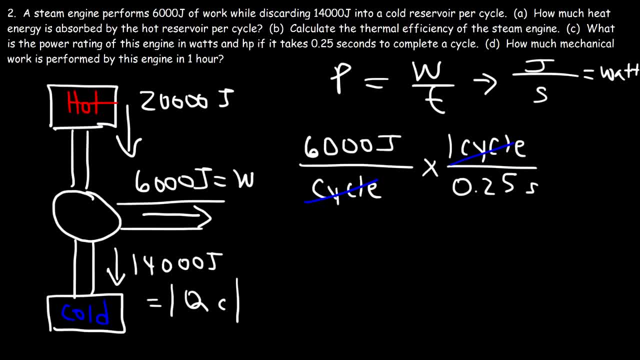 So if we set up this way, notice that the unit cycles will cancel And this is going to give us the unit joules per second, which is equivalent to a watt. So it's 6,000 joules divided by 0.25 seconds. 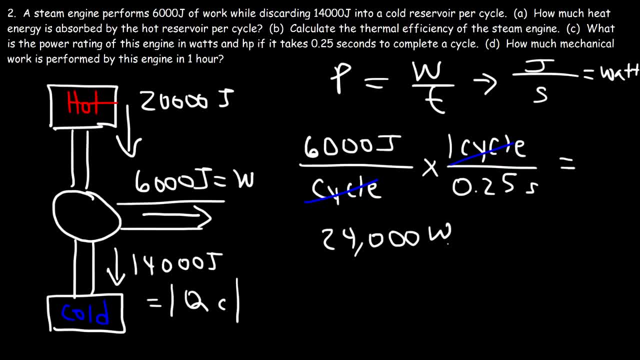 So the power rating is 24,000 watts. So that's the first answer to part C. Now we also want the power rating in horsepower, And you need to know that one horsepower is equivalent to 746 watts, So 24,000 divided by 746.. 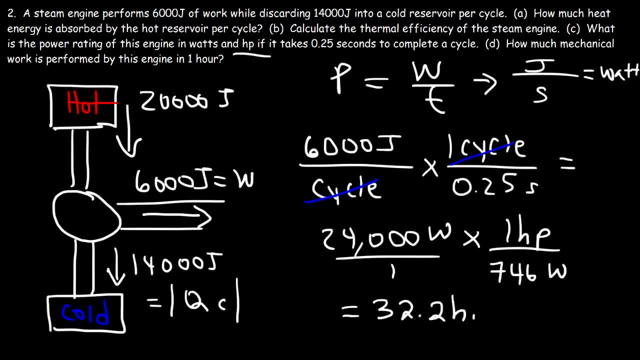 And so this is equal to 32.2 horsepower. So that's the power rating of this particular engine, or steam engine. Now how much mechanical work is performed by this engine in one hour? So how can we get that answer? Well, we need to do is start with the power rating. 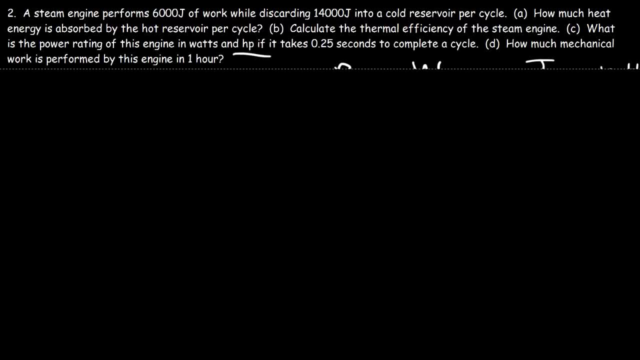 But first let me get rid of some stuff. We said that the power rating is 24,000 watts, which is equivalent to 24,000 joules per second, But actually I'm going to start with hours, So the time is one hour. 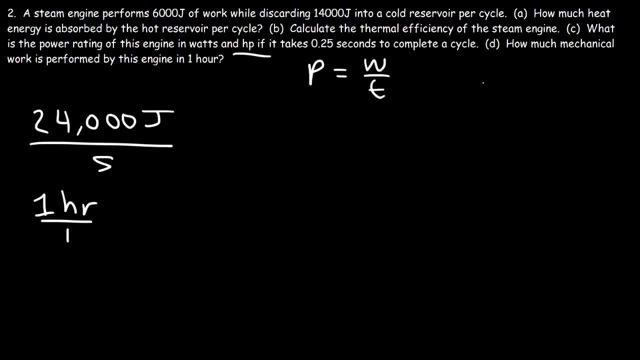 Now we know that power is work divided by time. So if you rearrange the equation, work is power multiplied by time. So I'm going to convert hours into seconds. One hour is 60 minutes And in each minute there are 60 seconds. 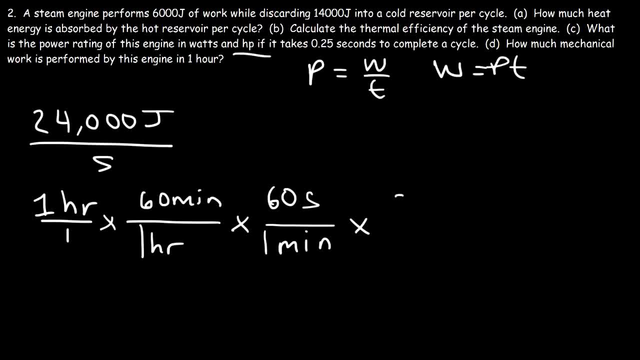 So now I have the time in seconds, I'm going to multiply it by the power rating, which is 24,000 watts or 24,000 joules per second. So the unit hours will cancel. The unit minutes will cancel. 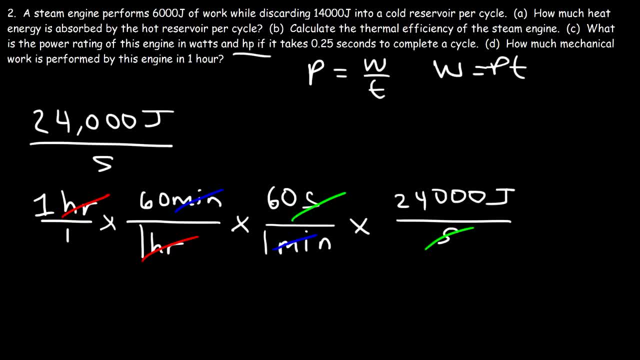 And also the unit seconds. The units will cancel as well. So this is going to give me the mechanical work performed by this steam engine in one hour. So it's 60 times 60 times 24,000.. So that's going to be a very big number. 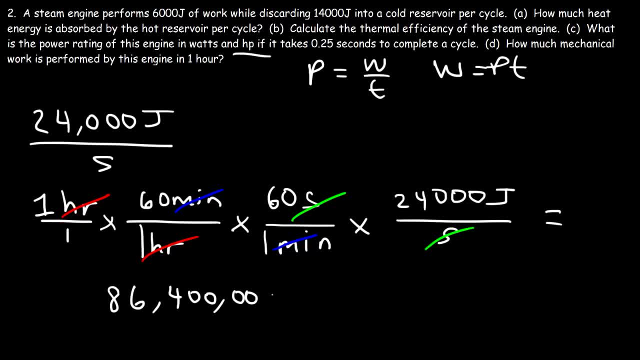 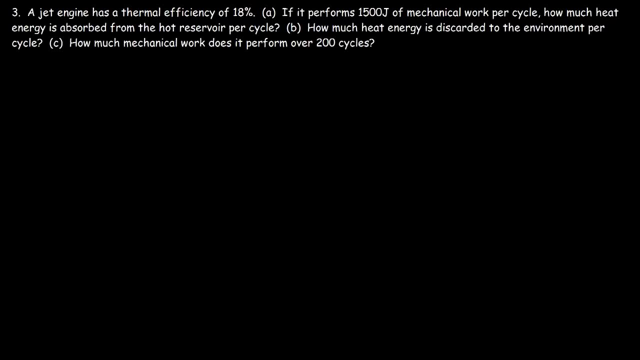 So it's 86,400,000 joules, Or you can write it as 8.64 times 10 to the 7 joules. So that's how much mechanical work can be performed by this steam engine in just one hour. 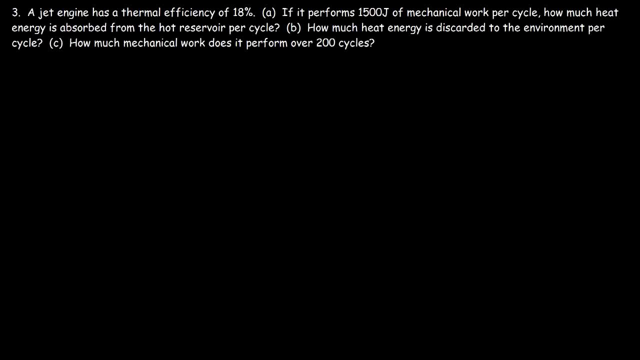 Number three: a jet engine has a thermal efficiency of 18% If it performs 1,500 joules of mechanical work per cycle. how much heat energy is absorbed from the hot reservoir per cycle? So we need to calculate QH. We have the mechanical work W and the efficiency E. 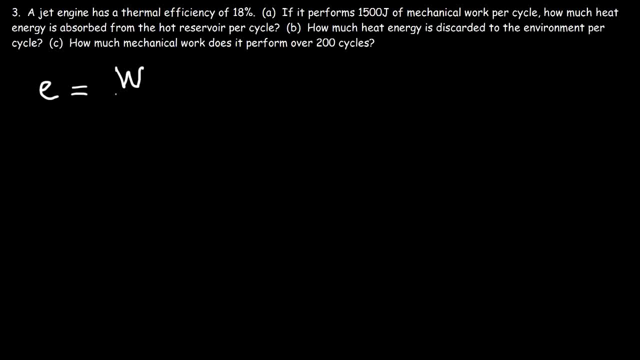 So we need to use this formula: efficiency is equal to the mechanical work Divided by QH multiplied by 100%. So the efficiency is 18%. The mechanical work is 1,500 joules, So the first thing we should do is divide both sides by 100%. 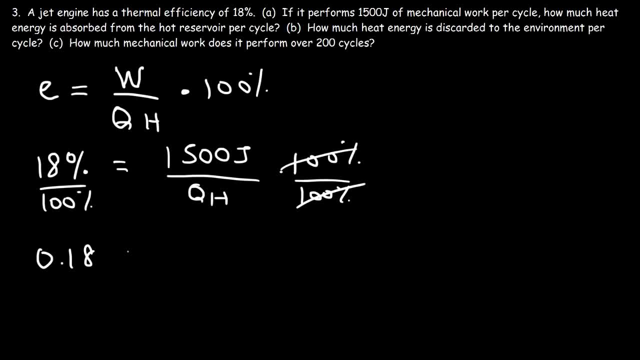 So 18% divided by 100% is 0.18.. And that's equal to 1,500 divided by QH. So at this point we can cross multiply. So this is going to be 1 times 1,500, which is 1,500. 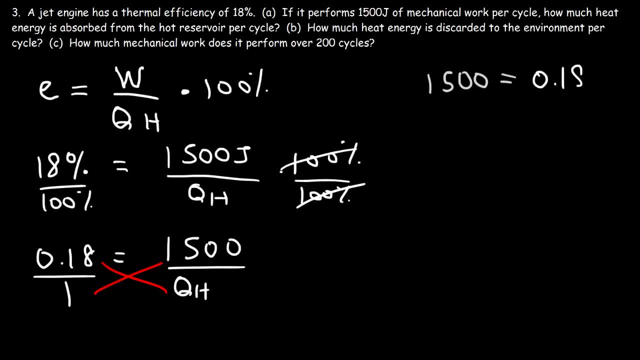 And then that's going to be 0.18 times QH. So to calculate QH we need to divide both sides by 0.18.. So QH in this example is 1,500 divided by 0.18,. 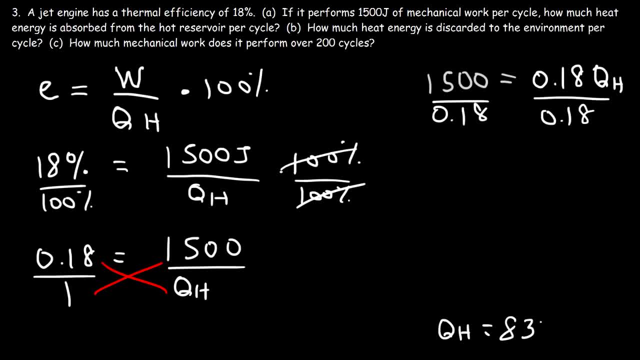 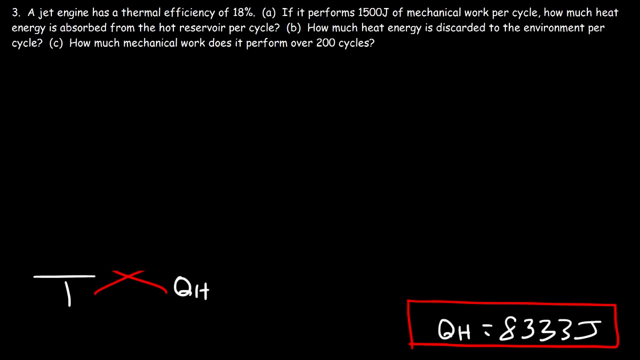 which works out to be 8,333.3 joules. I'm just going to round it to the nearest whole number, And so this is the answer for part A. Now let's move on to the next part. How much heat energy is discarded to the environment per cycle? 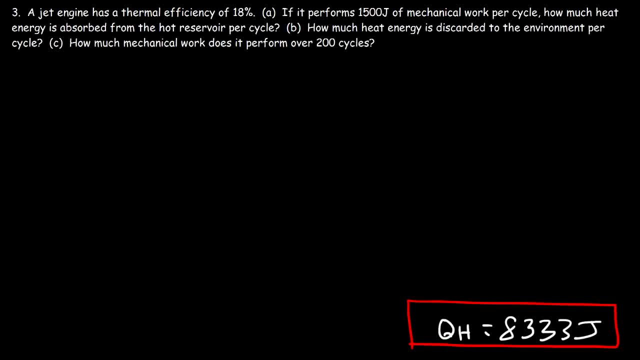 That was not supposed to happen. So we need to calculate QC. So we know that W is the difference between QH and H. So we know that W is the difference between QH and H. So we need to calculate QC. So we know that W is the difference between QH and H. 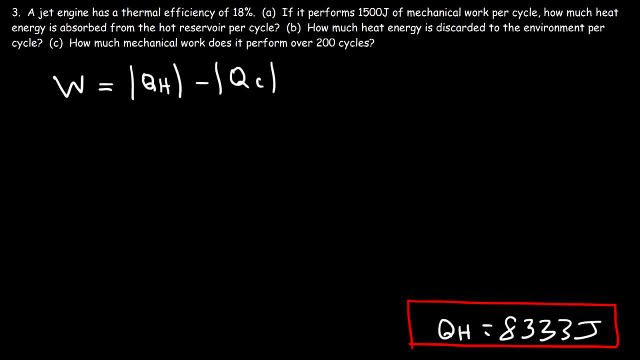 W, the mechanical work is 1,500, QH is 8,333. And so to calculate QC, what we need to do is basically subtract both sides by 8,333.. So 1,500 minus 8,333, that's negative 6,333 joules. 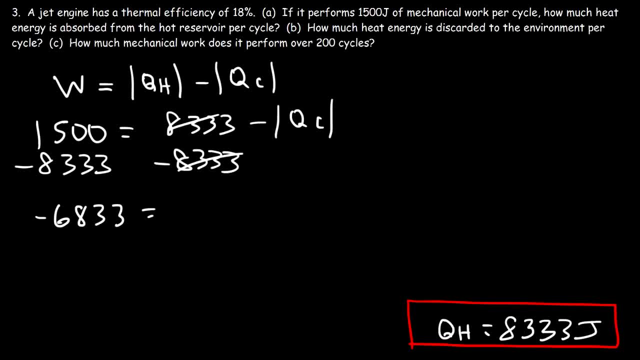 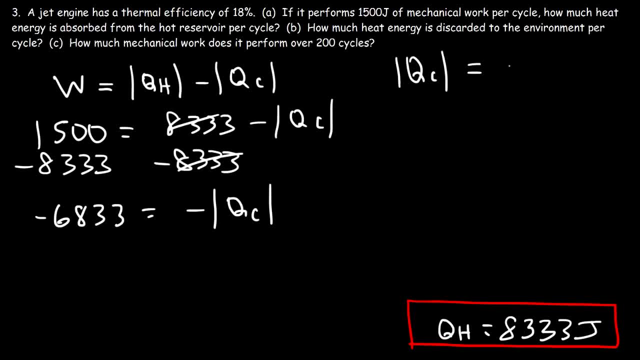 So we can see that the absolute value of QC is 6,833 joules. So that's how much heat and energy is discarded to the environment. Now, if you want the actual value of QC, keep in mind that it's really negative because the heat engine 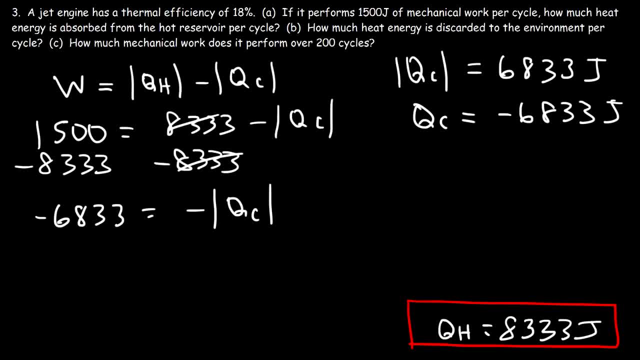 or the jet engine releases that heat. That's an exothermic process And any time the system releases heat energy in that process is negative for Q. but if you're not worried about any negative signs, you could say that 6833 jewels of heat energy was discarded. now let's move on. 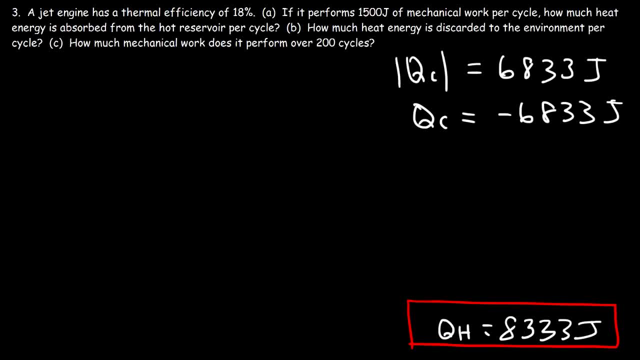 to Part C. how much mechanical work does it perform over 200 cycles? now keep in mind that it's 1500 joules of mechanical work per cycle, so all we need to do is take this value and multiply it by 200 cycles. so 1500 times 200, that is equal. 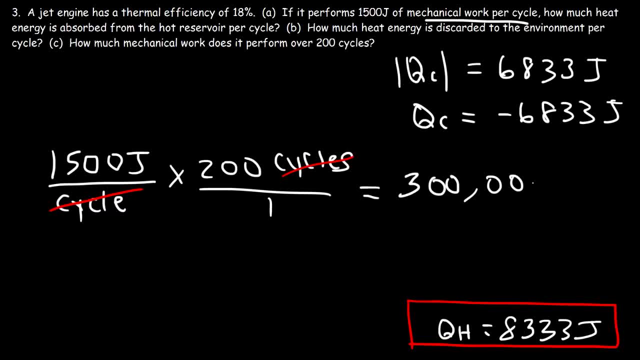 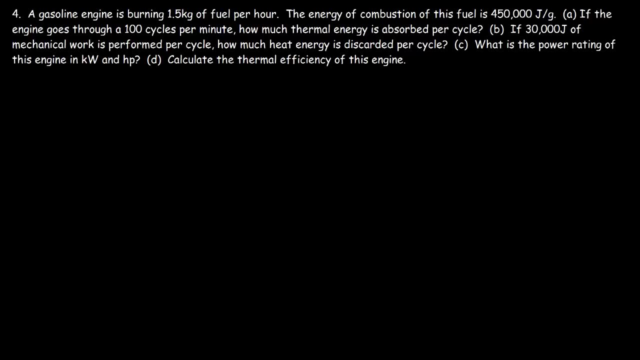 to 300,000 joules. so that's how much mechanical work the jet engine performs over the course of 200 cycles. and so that's it for this problem number four. a gasoline engine is burning 1.5 kilograms of fuel per hour. the energy of combustion of this fuel is 450,000 joules per gram if the engine 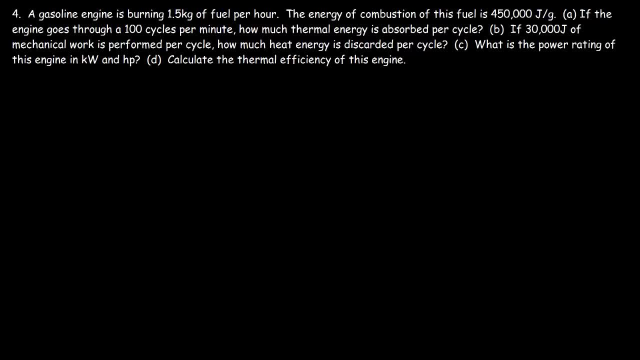 goes through a hundred cycles per minute, how much thermal energy is absorbed per cycle? now our goal is to calculate the energy per cycle, so we need to perform a unit conversion process. to calculate the energy per cycle, so we need to perform a unit conversion process and our goal is to get joules on top and the number of cycles on the. 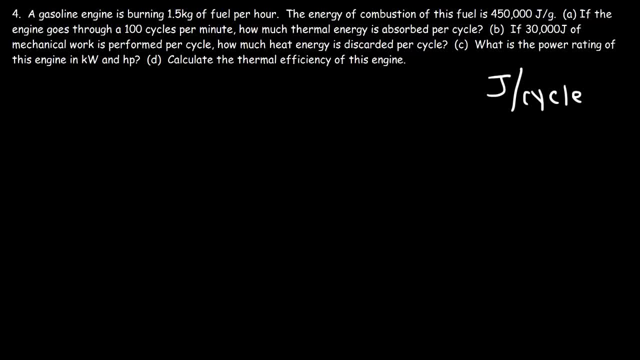 bottom. so I'm going to start with the rate at which the fuel is burned. so 1.5 kilograms of fuel is burned per hour, so we need to write it like this now: the combustion is joules per gram, so that indicates that I need to convert. 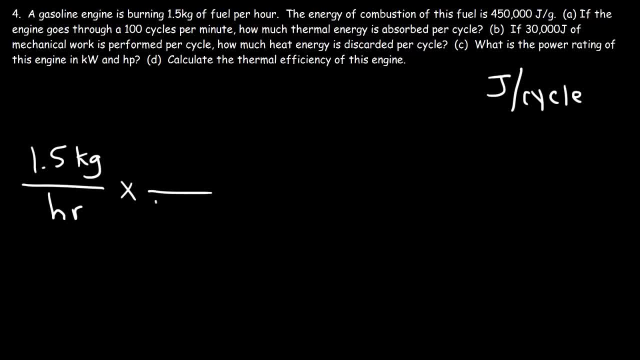 kilograms to grams. so one kilogram is equal to a thousand grams of fuel per gram, and so we can cancel the unit kilograms. so now I can use this value to convert to joules. so the energy of combustion is 450,000 joules per gram now. 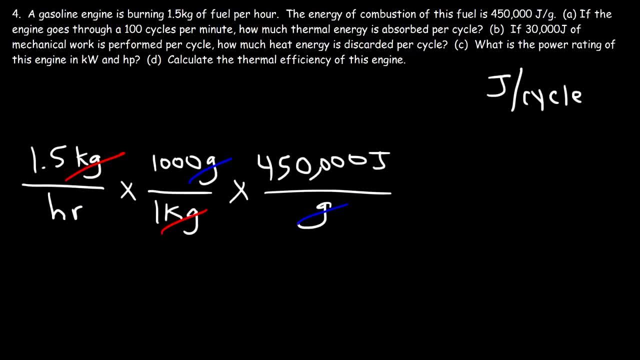 I still have a unit of time that I have to get rid of, and this value connects cycles with time, so I have a hundred cycles per minute, which means I need to convert hours into minutes. so one hour is equivalent to sixty minutes, so the last thing I need to do is 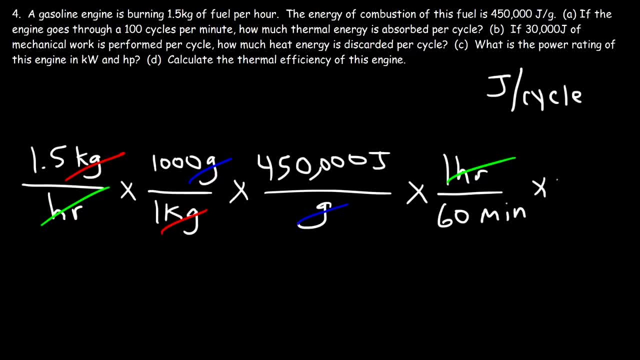 multiply by the number of cycles per minute. so in one minute there are a hundred cycles. so we can cancel these units. so now I have the energy in joules per cycle, so it's going to be 1.5 times a thousand times 450,000, divided by 60, and 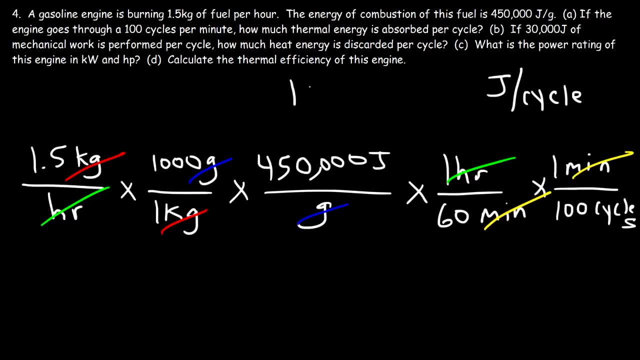 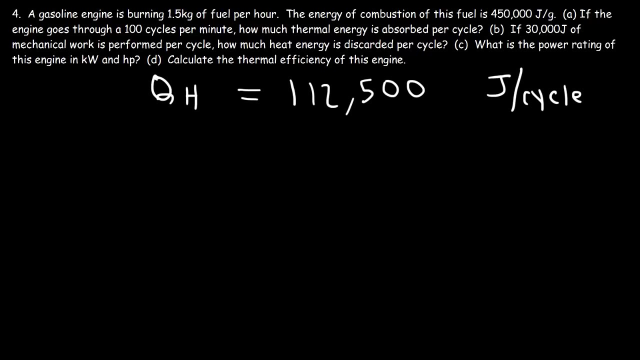 then divide that by a hundred, so this comes out to be a 112,500 joules per cycle. now, because the thermal energy is absorbed by the engine, this has to be qh, and so that's it for part 8. Now let's move on to part B. If 30,000 joules of mechanical work is performed per cycle, 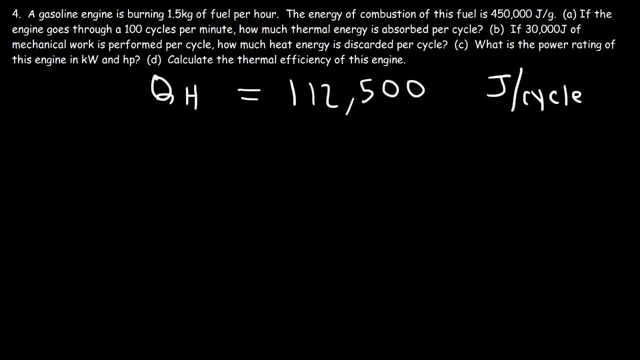 how much heat energy is discarded per cycle. So we know that W is equal to QH minus QC. So our goal is to calculate QC. So let's rearrange the equation. I'm going to take this term and move it to this side, where it's going to become positive. 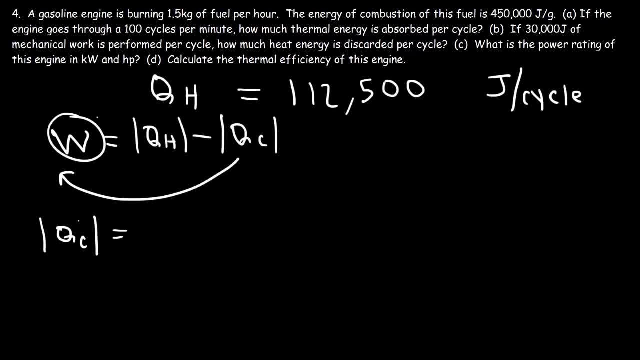 QC, And I'm going to take W- move it to that side where it's going to be negative W. So this is how we can calculate QC. So QH is 112,500 joules per cycle and the mechanical work is 30,000 joules per cycle. 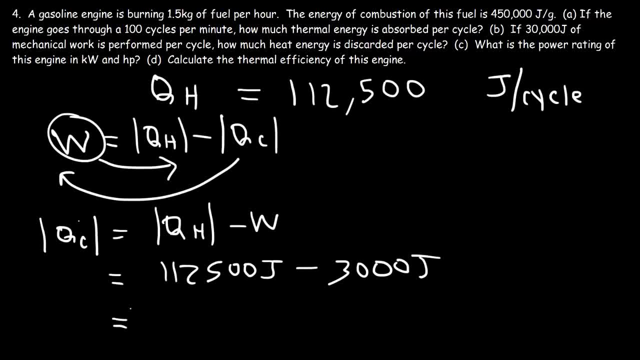 So if we subtract these two numbers, Okay, So that's 12,500 joules per cycle. This will give us 82,500 joules, and I need the extra zero. That's supposed to be 30,000 as opposed to 3,000.. 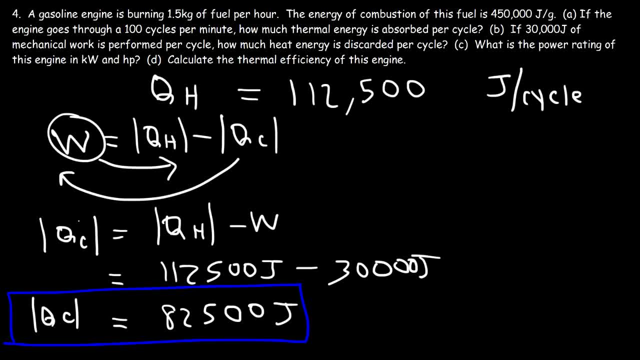 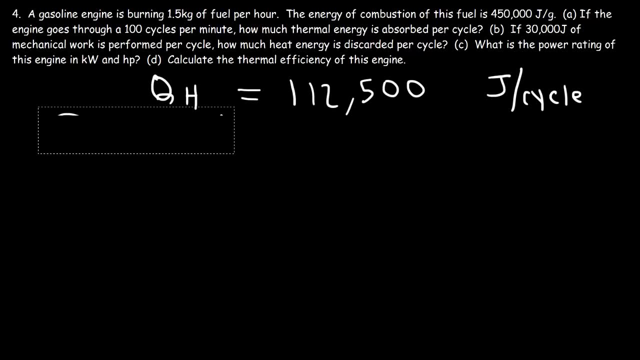 So this is the answer for part B. Now let's move on to part C. What is the power rating of this engine in kilowatts and horsepower? So how can we get that answer? We know that power is work divided by time, and we have the mechanical work. 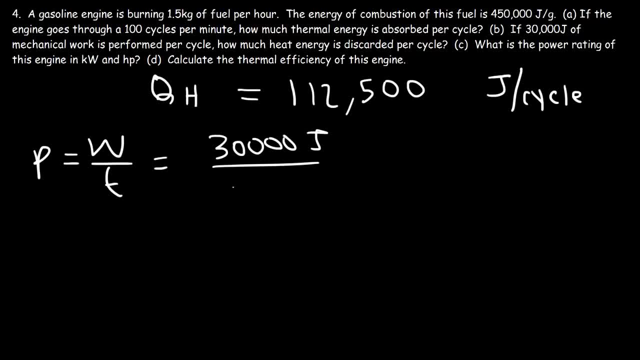 It's 30,000 joules per cycle and we have the time it takes to complete one cycle, which is currently 100 cycles per minute. Okay, So let's multiply it by that. Now we need it in second stone, because one watt is one joule per second. 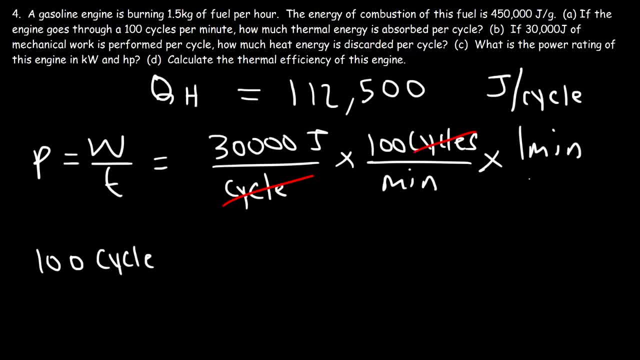 So let's convert minutes to seconds. One minute is equal to 60 seconds, So it's going to be 30,000 times 100 divided by 60. And so the power is 50,000 watts. Now to convert that to kilowatts we need to divide it by 1,000..